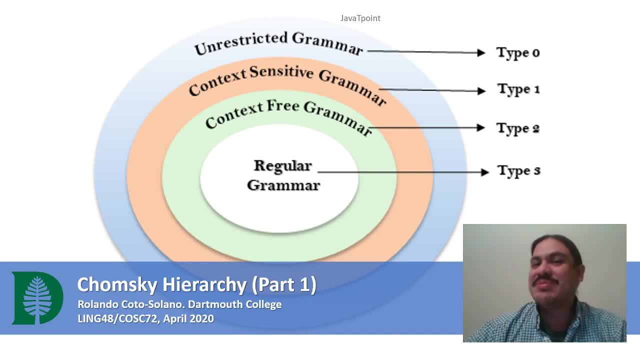 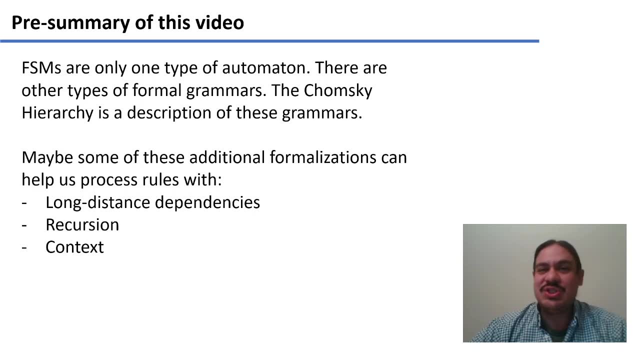 Let's do this. Let's talk about theory of computation and the Chomsky hierarchy. So we've been talking about finite state machines. Finite state machines are a kind of abstraction of what a computer program does, If you think about them going from state to state with a transition. 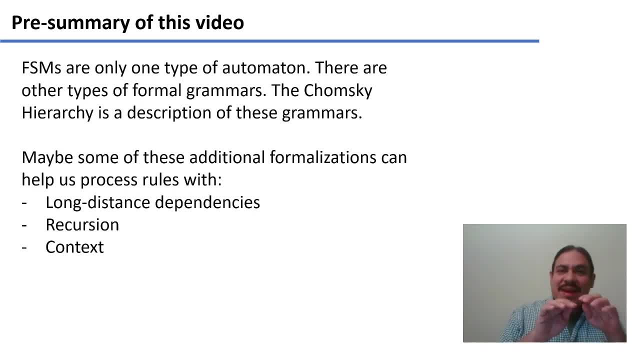 is sort of similar to saying: if something happens, then do something else. If I get this input, then perform this output. This finite state machine is an abstraction of what a computer program can do, and it is only one type of abstraction. There's many other ways to explain. 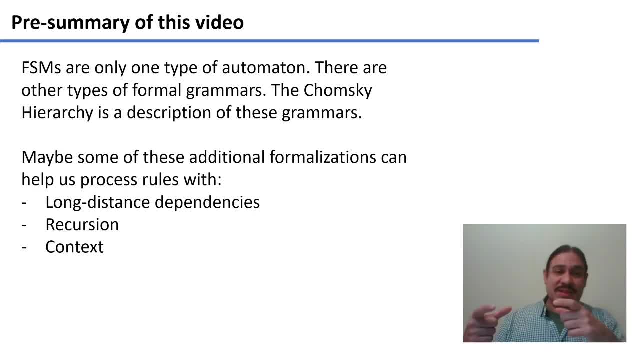 what computer programs can perform on strings, the kinds of operations they can perform, and we call these formal grammars. The Chomsky hierarchy is a description of these grammars, from most restrictive, which is what we've been seeing so far, finite state machines, to most powerful, which is Turing. 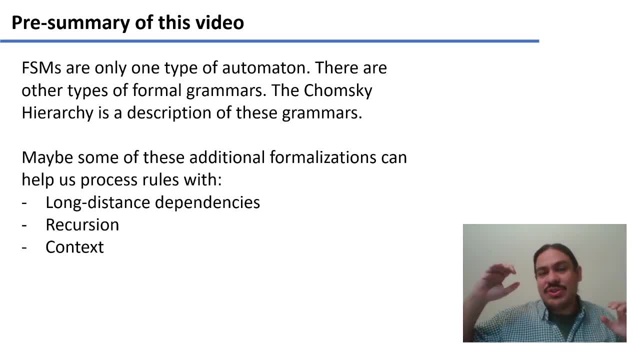 machines which essentially can generalize to performing any operation on a string. Some of these formal grammars are going to help us overcome the difficulties that we've had, For example the fact that some things in language have long distance dependencies where two distances 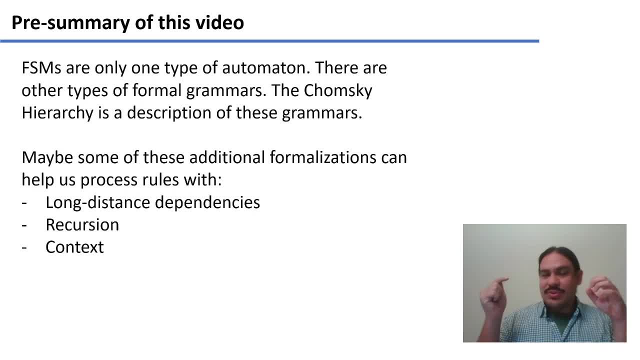 and states have to communicate with one another in order to work. They can help us overcome the problems of recursion, where our finite state machine has to keep going down, and down, and down and then remember the path upwards, and upwards, and upwards, so that it goes down n times. 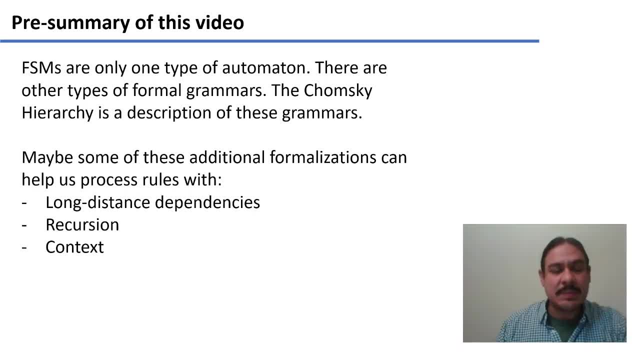 and then it comes back up an equal n number of times. Likewise, they can help us with the problem of context, where, before you apply a rule, you need to figure out what other symbols there are around you and, depending on those, you perform the rule in one way or the other. 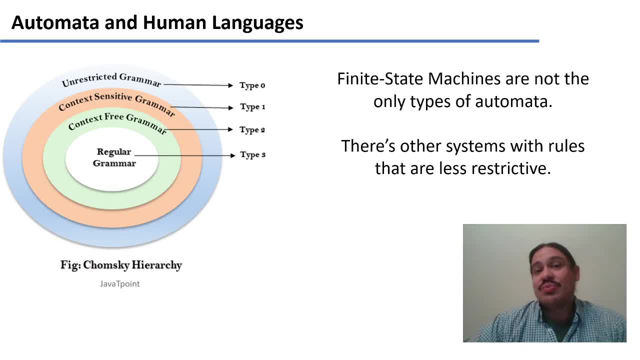 So again, finite state machines are just one type of automaton, and there are other systems that are less restrictive and they are here in the Chomsky hierarchy. Type three is a regular grammar, which is the kind of grammar that a finite state machine can. 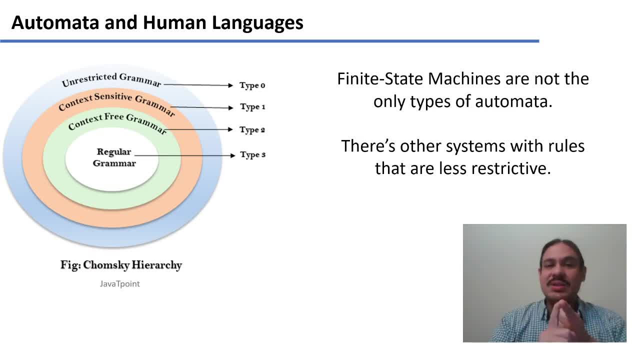 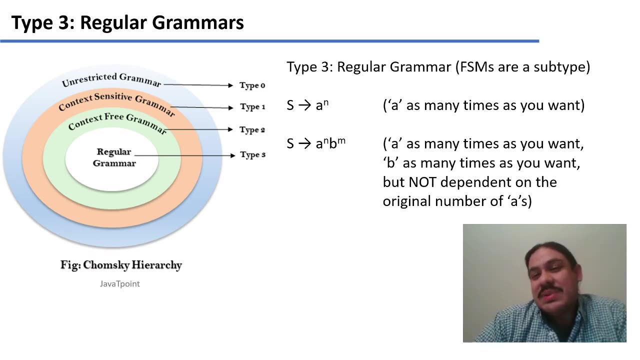 describe. we have other types of grammars: Context-free, context-sensitive and unrestricted, or computationally innumerable. Let's look at each one of them. A type 3 grammar or regular grammar is what we have been seeing so far. A. 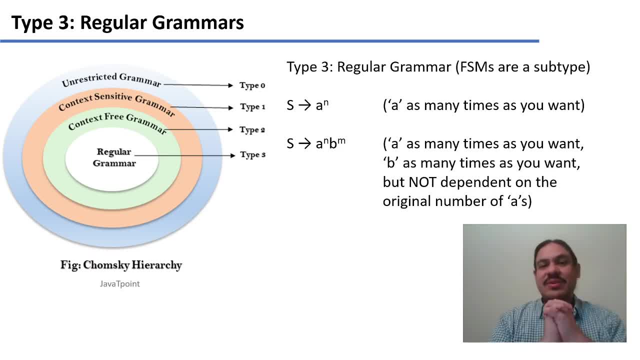 finite state machine is a subtype of regular grammar. You can have a rule that has one input, where you have one task that you want to perform: create a sentence. You don't need to look at the sentence before or after to perform the task. You only want to create this sentence here And you create the. 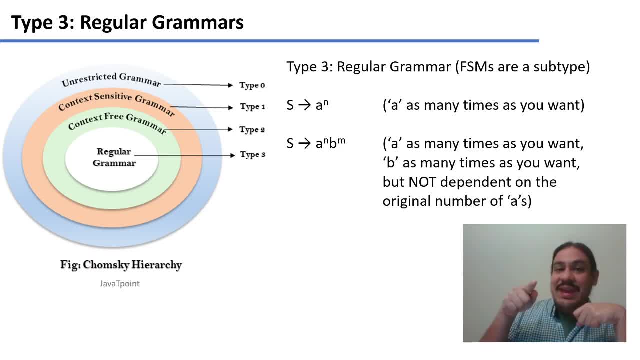 sentence by making the symbol a n times or having many symbols n times, n times, But there's no way for you to create a sentence that has one input where you can coordinate that these two run at the same time. Each state is independent of each other in how many times it executes. This is the grammar of the. 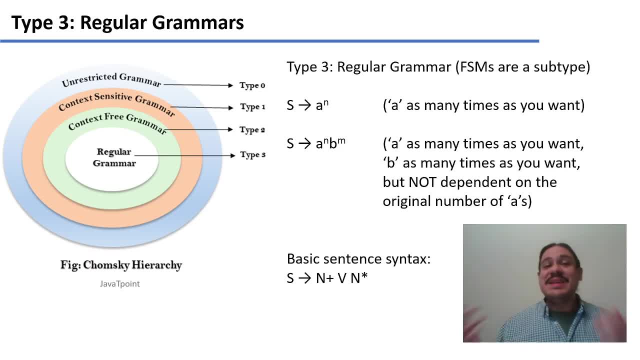 basic structures that we had so far, Like Jane eats pizza, One noun for the subject, one verb and 0 or more nouns for the direct object. English sentences. In English sentences, the number of nouns for the subject and the number of nouns for the direct objects are not connected. If you have, James. 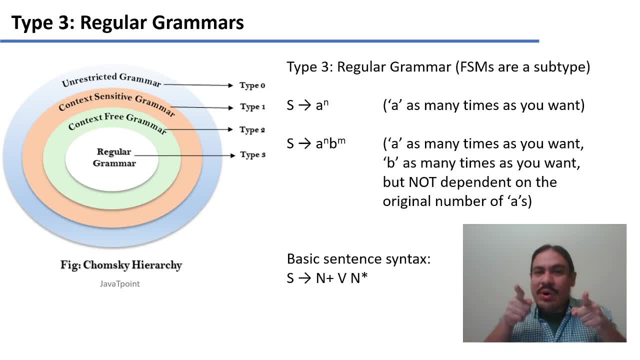 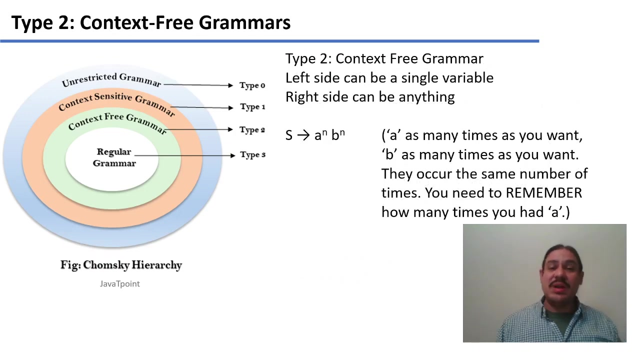 Smith. here you do not need to have two words in the direct object- James Smith eats pizza, where this is two and this is one is a perfectly valid English sentence. So this is a type of rule that would be described through a regular grammar. Let's look at a context-free grammar. This is one where 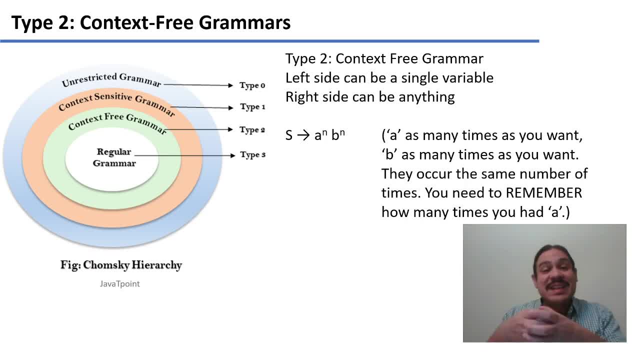 you have a single variable going in. you know you want. you want to generate a sentence and then the output, or the right side of the rule, can be anything. You can have more than one symbol. These symbols can coordinate how many times you run them, but then you would need to program something to help them remember. 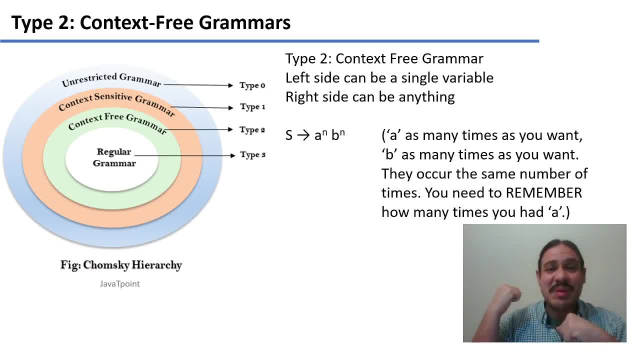 It can be a variable somewhere that remembers that n is equal to 3.. It can be a data structure like a push-down stack, where if you push a n times, then you know you have to pop a n times, and so the popping could be the number of times you run b. So if you pop a 1,, 2,, 3,. 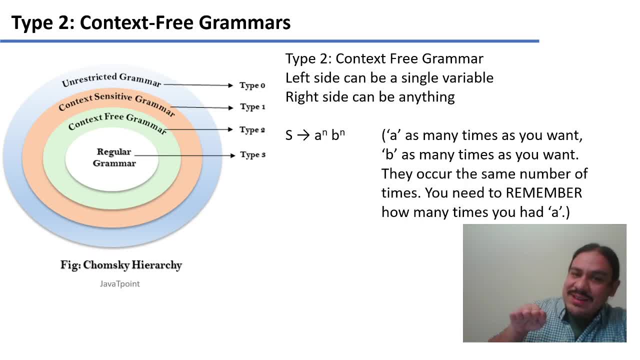 and then I'm sorry if you push them 1,, 2,, 3, and then you know you have to pop them 1,, 2,, 3, this could be the number of times you have b, b, b, b, So as you can, 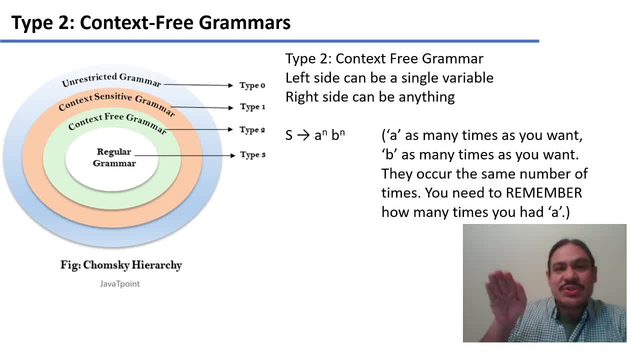 see, you can implement memory with a structure like a push-down stack and you can implement it with a variable. There's something that you'll have to do that is additional to the description of the states and their transitions. This is, of course, going to cost you computationally. One rule that can 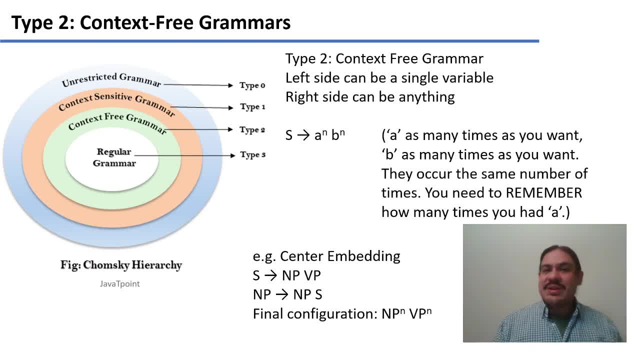 be explained with a context-free grammar is center embedding, For example, the sentences like the cat that I like eats a tuna, where you have a sentence like the cat eats tuna and then the noun phrase can also have a sub-sentence- The cat that I like eats tuna. for example, In the 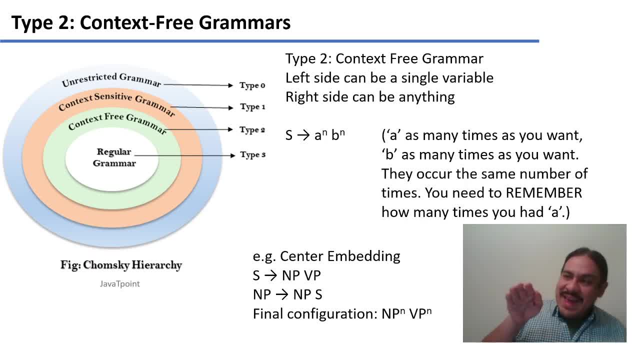 final configuration. you need cat, cat I and then like eats, So you need to push two nouns and then pop two verbs. Or you can just have a variable that remembers that n is equal to 2 and tracks that you have two nouns going in and two verbs going out. This is 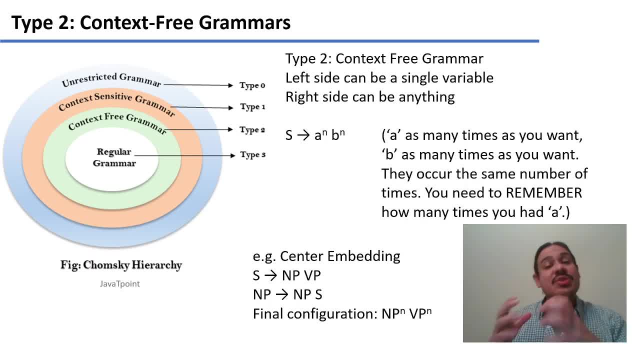 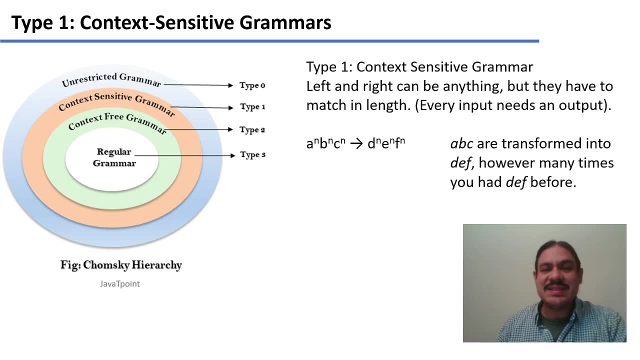 a context-free grammar. And again, it's context-free because, in order for you to construct your sentence, you do not need to look at previous sentences or at following sentences. A type 1 grammar is a context-sensitive grammar. In these kinds of rules, you can have anything on the left side and anything on the right side. 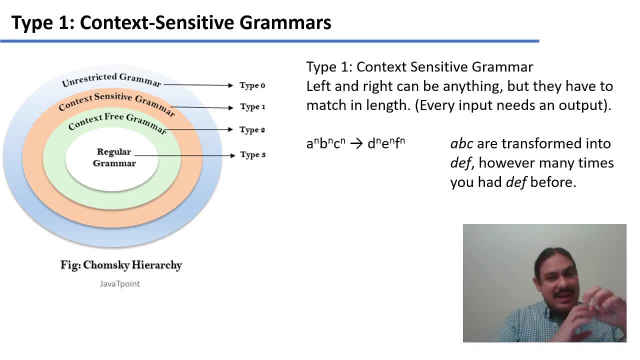 But you do need to have, for every input, an output. For every time, for every element, like a to the n, you need to output something. It might be the same or it might be different. For example, in the Yoruba emphatics we have a rule that took a vowel, a tone. 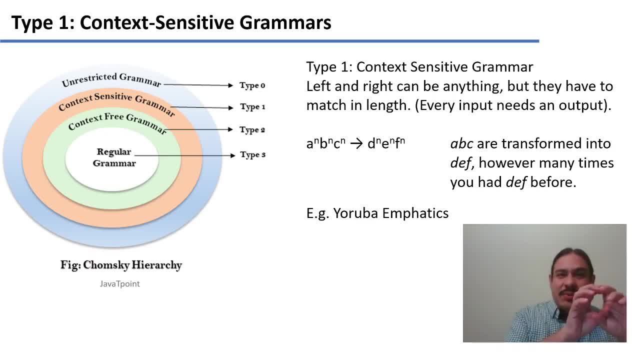 and a consonant if it existed. For every vowel you had in the input, you had to produce the vowel in the output. For every consonant you had in the input, you had to bring the consonant to the output. But then for every tone in the input, you had to read it. you had to perform an operation. 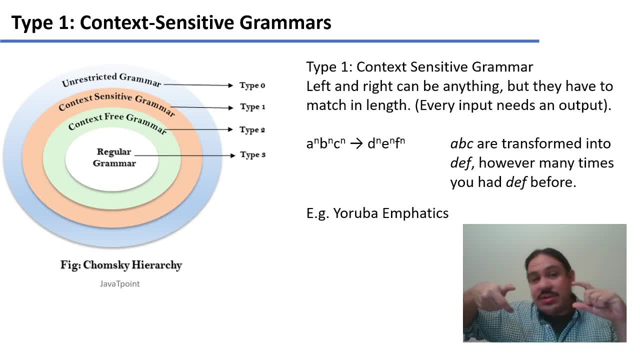 on it and you had to give us an output. So there's a one-to-one correspondence, even if the output itself is different. We call it context-sensitive Again. context-sensitive because in order for you to know what D E, F is, you need to read some. 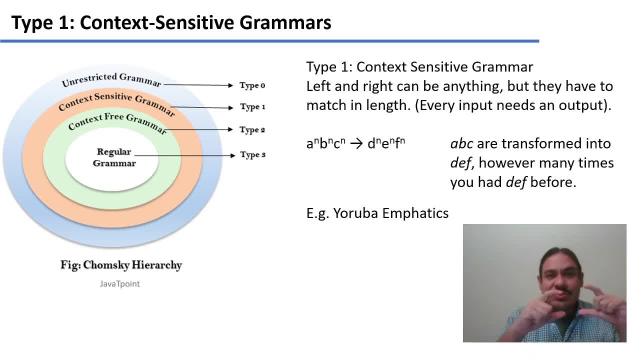 things about A, B, C And in order for you to know what A, B and C, how A, B and C are going to interact, you need to actually look at them, to look at the sounds before and after you. 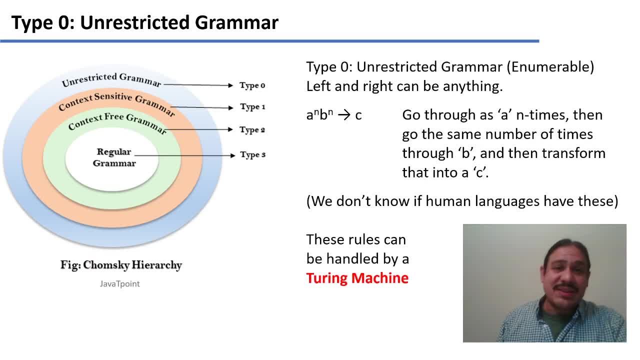 So regular grammars are, for example, a basic English sentence. Context-free grammars are more complex and you need to coordinate things, but you still don't need to look at sentences around you. A context-sensitive grammar is one where you do need to look at the sounds around you, like in Yoruba tones. 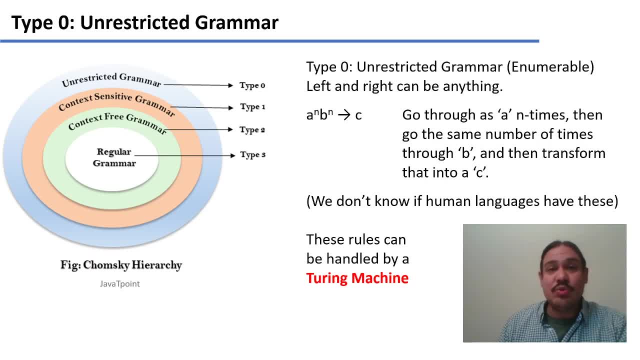 And an unrestricted grammar or a computationally enumerable grammar is anything else, One where you can have an arbitrary number of symbols at the input and then produce some output that is not necessarily matched to the input. Human languages probably don't have these kinds of rules, but this is the kind of rule that can be handled by a Turing machine. 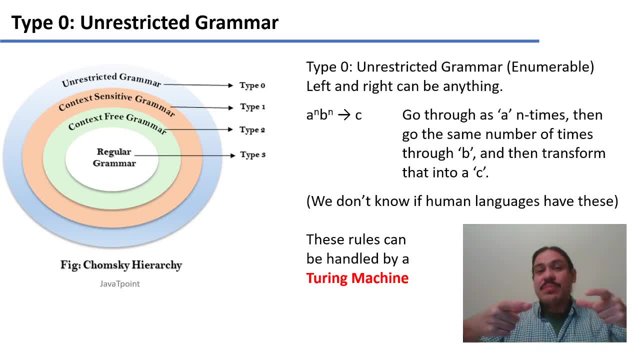 A Turing machine would take a string, an input string of any kind, an arbitrary number of symbols, and then it would transform it into some other string with an arbitrary number of symbols in the output. Of course, the problem with this is that this comes with added computational power. 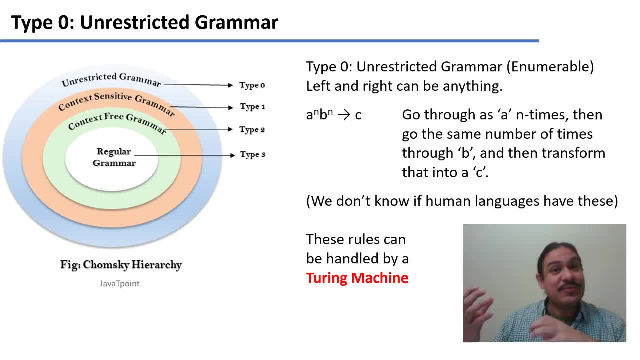 We can take any input. We can take any input and put it into any out and convert it into any output. But now the cost is that not only is our processing going to skyrocket, we cannot even guarantee that we're ever going to stop the operation. 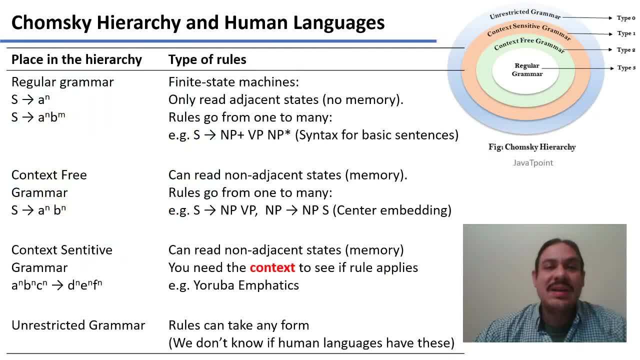 More on this in the next video. In summary, we have four main types of grammars for the Chomsky hierarchy. We have regular grammars, which take one input and have many outputs. These outputs are each of them independent from the other and they don't remember how the other behaved. 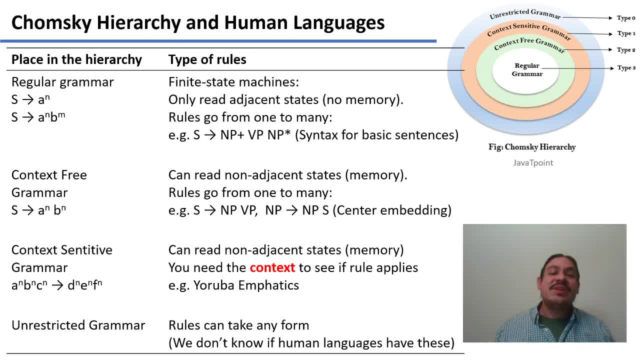 This is our syntax of sentences. in English We have context-free grammars where we have one input, doesn't need to look at the context, and we can have many outputs, and these outputs can communicate with one another And we would need to implement some computational way for them to communicate- a push-down stack, for example. 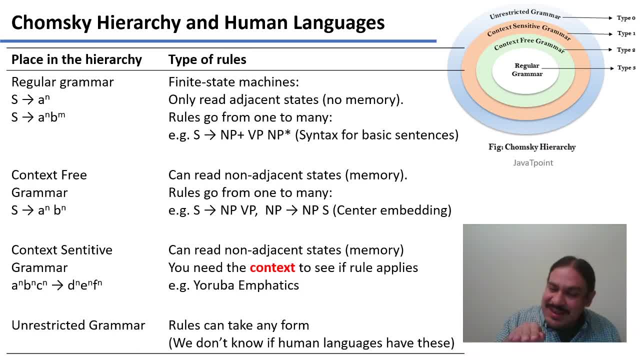 So we know that we push so many in and we need to pop so many out. A context-sensitive grammar would be one that takes an arbitrary- I'm sorry that takes input, and then for every input you need to write an output. 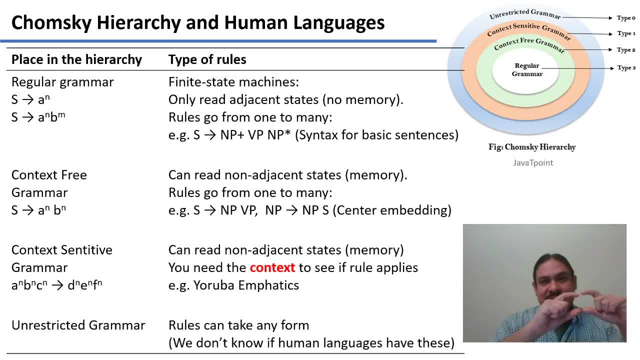 You can transform symbols and, with this, make the rule context-sensitive, because you need to look at them in order to know what you're doing. But you need to provide for every input an output. Finally, an unrestricted grammar is one where the rules can take any form. 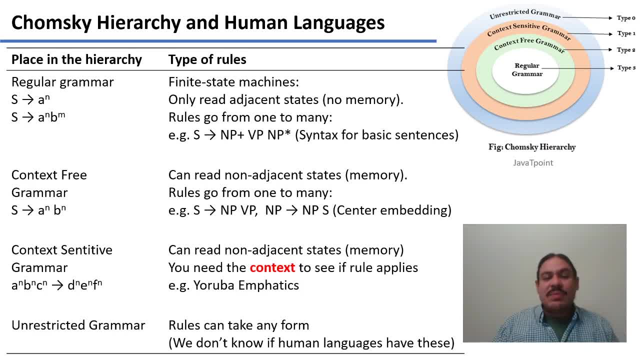 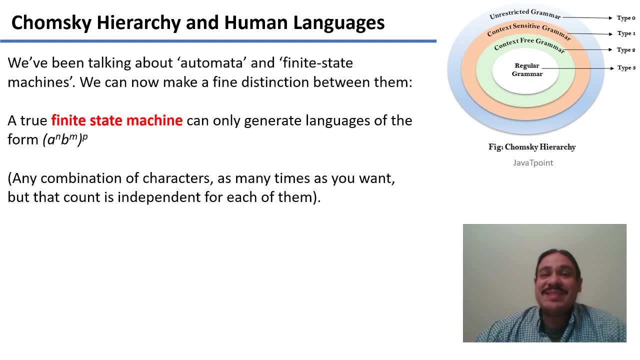 You can take any string and transform it into any other string. Human languages probably don't have these, but this is the kind of rule that we actually do need in computer science, for example, So we can finally make the definition very precise. Finite state machines are a kind of automaton. 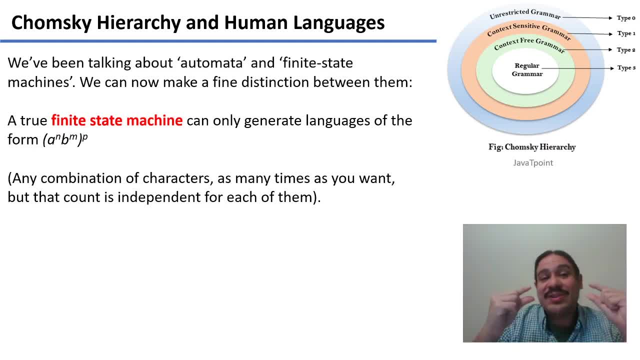 A finite state machine is one that It generates regular languages in the form, for example, A-N, B-M, P. You can generate an arbitrary number of symbols, an arbitrary number of times, but they're not going to be communicating with one another. 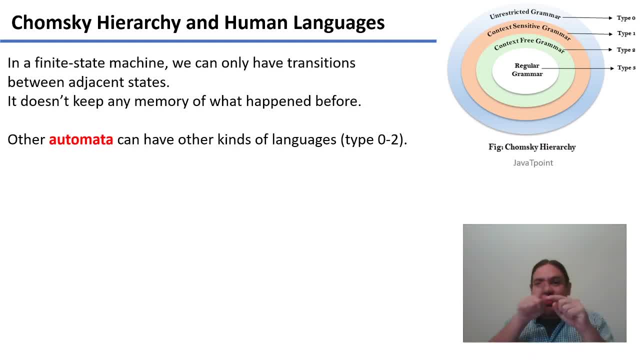 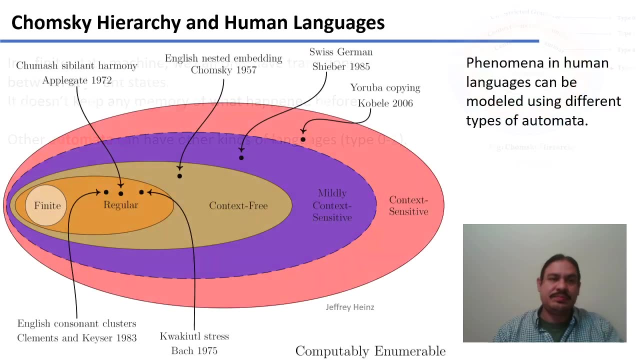 We can only have transitions between states, so you cannot have communications across distant states in finite state machines. You can have them In other types of grammars, but this is going to cost us computationally. This, by the way, is the same hierarchy, just displayed slightly differently. 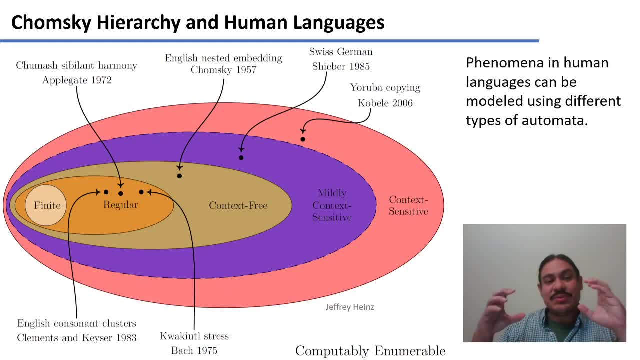 As you can see, we have, as in finite languages, is the most restrictive kinds of languages Within it. for example, we have logic like true or false statements. We have rules that are regular, That can be modeled by Finite state machines. for example, are English consonant clusters, have some structure to construct syllables, but we only need to look inside of our syllable to construct it. 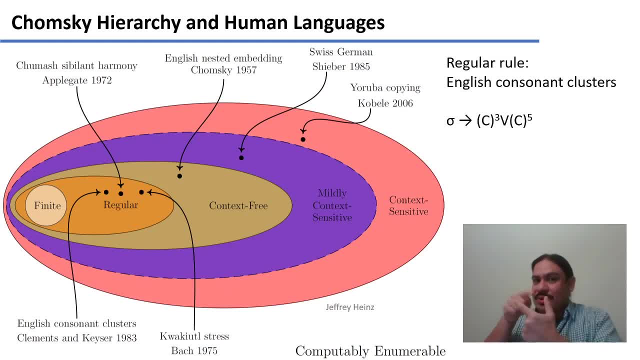 We don't need to look at other syllables to know what our syllable needs to look like. We have context free rules where you need to implement means for the computer to remember what it's doing, such as the stack, for example, or variables or some other way. 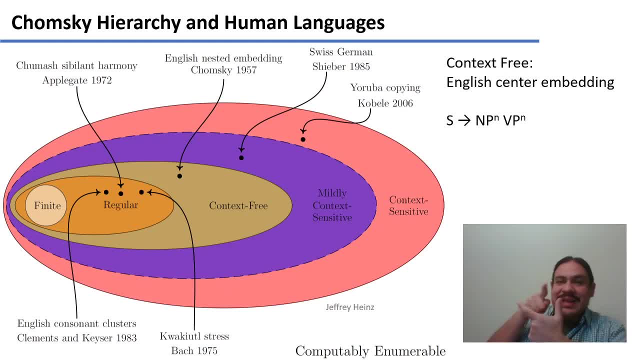 So that you can have as many and nouns and as many verbs as you need. but you still don't need to look at the sentences around you. We have at the outside edges of this hierarchy rule, like the Yoruba emphatic, Where you have a rule that takes the part of a syllable, reads it and then generates the output based on what it saw and its immediate content. 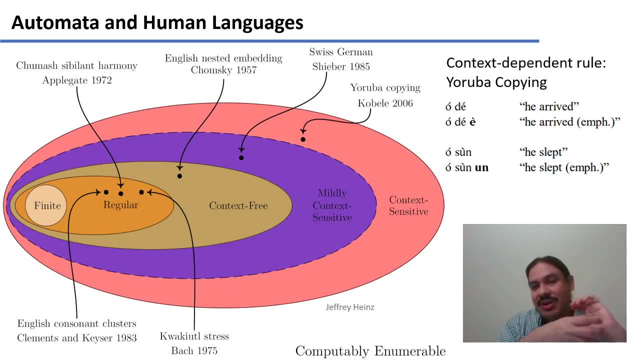 Let me just put it in the prerequisite: We gotра dog meets a dog. We got it We look for, Or Drum beats in its context, Not just immediate context, but it could be context several symbols away, several sounds away, Like in the second case. 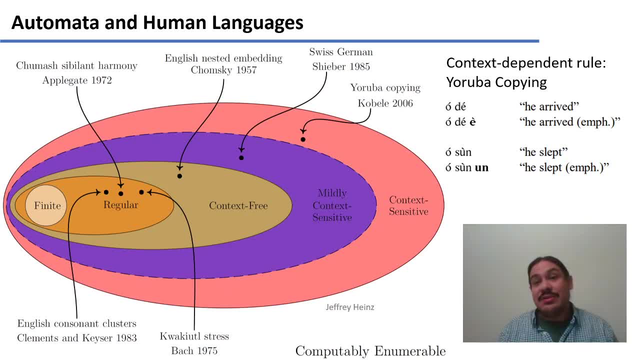 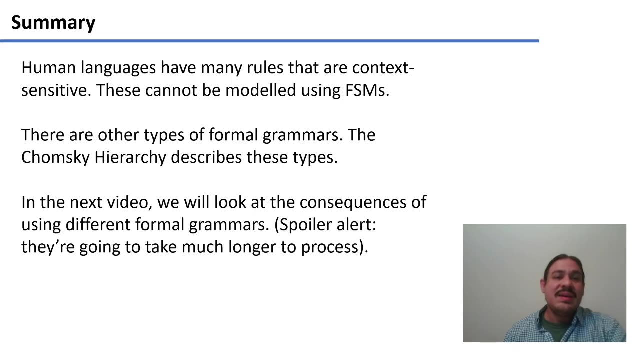 where you have to go not one but two back, and could potentially go even further back. And again, we don't know if human languages have rules that are more complicated than this. We would call those computationally innumerable rules. In summary, human languages do have rules that are context-sensitive and that cannot be modeled.